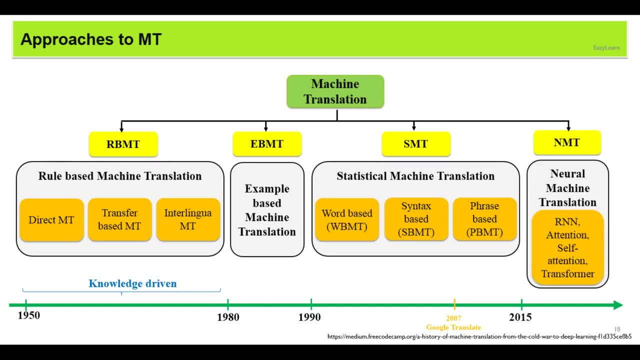 Here again, we have three different approaches. And then we have the neural machine translation. These three approaches are called the data-driven approaches or the corpus-based approaches. Here the system learns the machine translation from the corpus. In this series we'll be discussing the SMT and the NMT part. 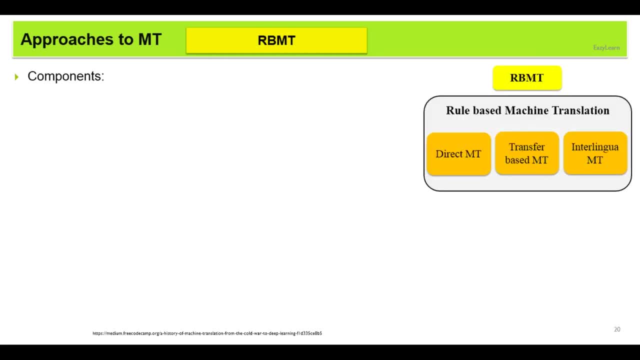 NMT is in much more detail. Now let's go through the RBMT, the rule-based machine translation. So in RBMT we have the three components. We have a bilingual dictionary. Let's see if we are translating from German to English. 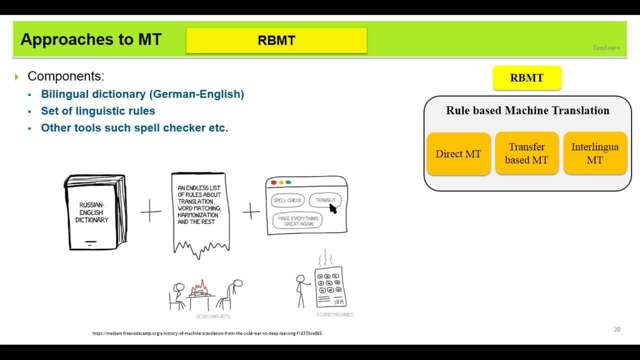 So we have a bilingual dictionary for German to English, We have a set of linguistic rules And we have other tools like spell checkers and all In RBMT. we again have three different approaches. One is direct machine translation, where we directly translate from the source language to the target language. 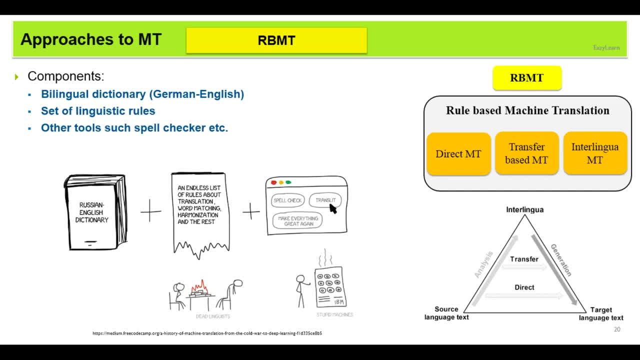 In the second approach, we first understand the grammatical structure of the sentence And then translate, And in the third one, which is called interlingua, we first translate the source language into a language-independent representation and then we translate it. 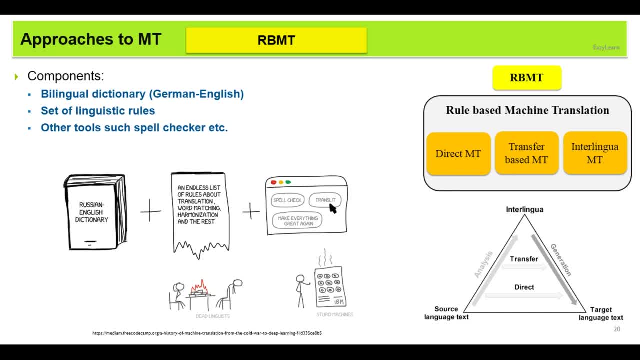 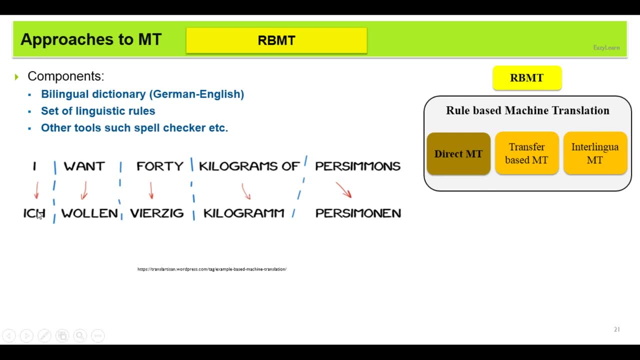 So we'll see the example of each of them in the later slides. So in the first one, we are directly translating this from the source language to the target language. In the second one, we first understand the grammatical structure of the source sentence, as I already said, 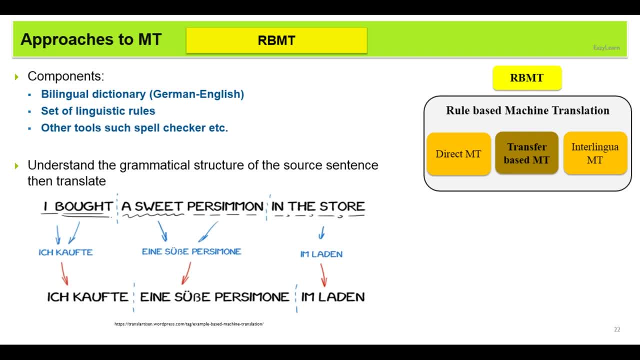 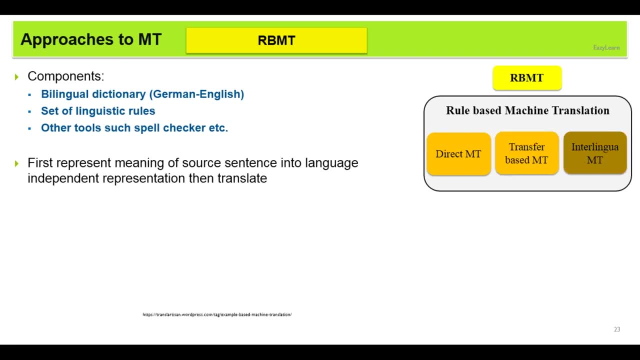 Like this, So we understand where is the subject, where is the object, what is the noun and all. So first we understand the grammatical structure like this, And in the third approach, we first, as I said, we convert it into a language-independent representation. 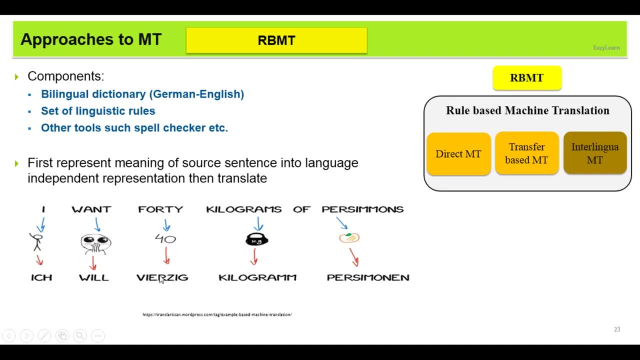 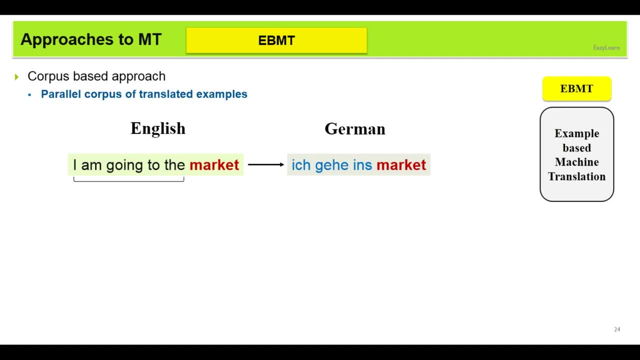 And once we get this, we can easily translate it to the target language- Now EBMT. So example based machine translation. Here we require a parallel corpus. So we have, let's say, if we are translating from English to German. 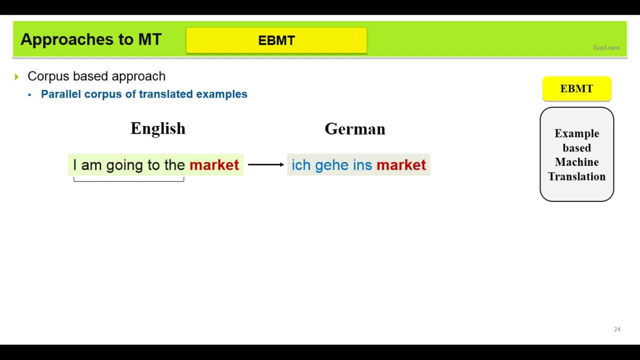 So we have a corpus. We have English sentences on the one side And we have the corresponding translated sentences in the German on the other side. So let's say, if we have a sentence, I am going to the market. So we also have a translation of this.